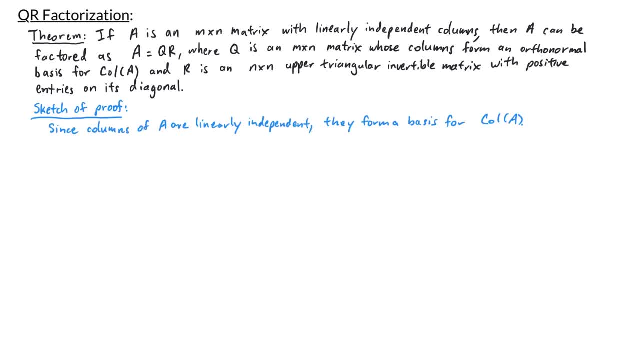 to Q and R. First of all, since A has linearly independent columns, I know that the columns form a basis for the column space of A. So if I want to find an orthonormal basis for the column space of A, all I have to do is use the Gram-Schmidt process on the columns. 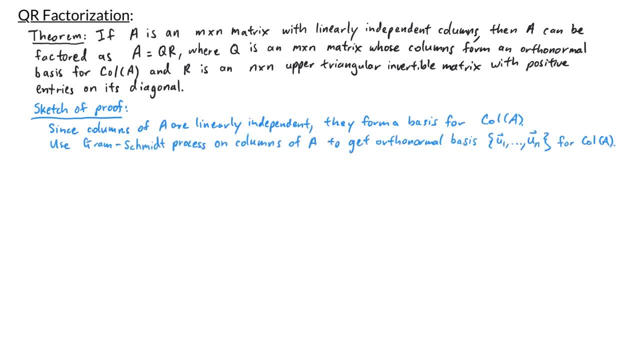 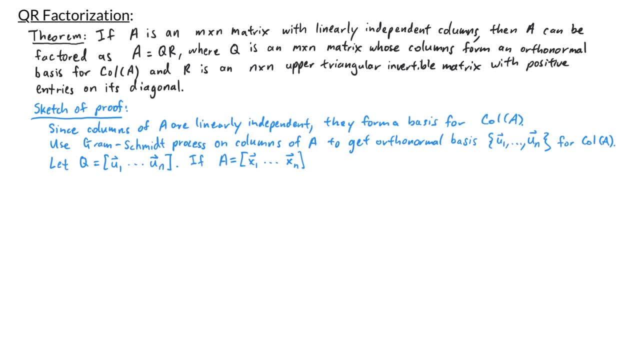 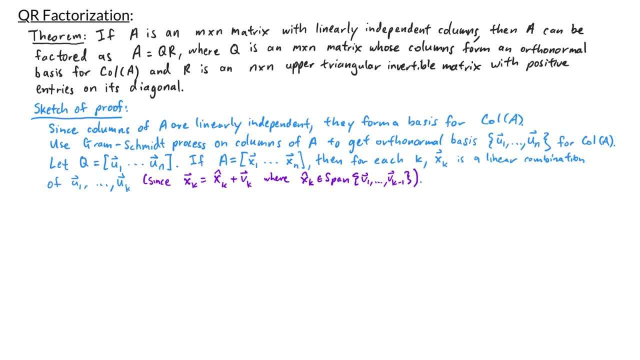 vk. Now x hat is in the span of v1 through vk-1, and so xk, being the sum of x, hat and vk, is in the span of v1 through vk-1.. vk, And since the vectors u are just the vectors v divided by their lengths, we have that xk is: 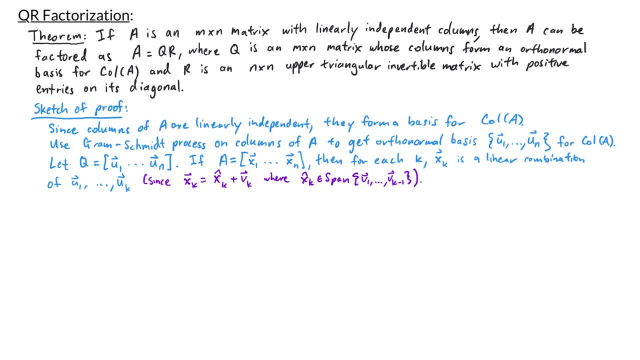 also in the span of u1 through uk. Now remember, if I want to write xk as a linear combination of u1 through uk, we know that the weights are xk, dot, the corresponding u vector. So we know we can write xk as xk dot u1 times u1, summed up through xk dot uk times uk. Now xk can also be thought of. 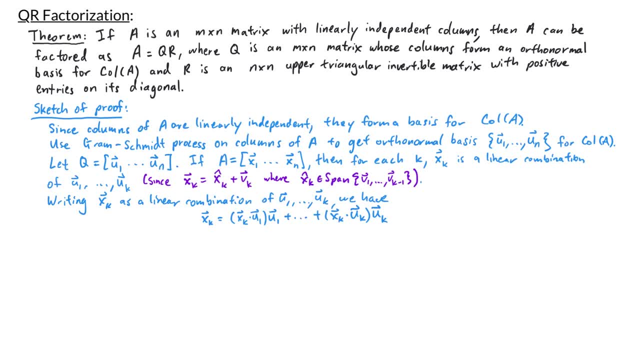 as a vector in the column space of a, which has bases u1 through un. So x can also be written as a linear combination of u1 through un. Now the unique representation theorem tells me that there's only one way to write xk: as a linear combination of u1. 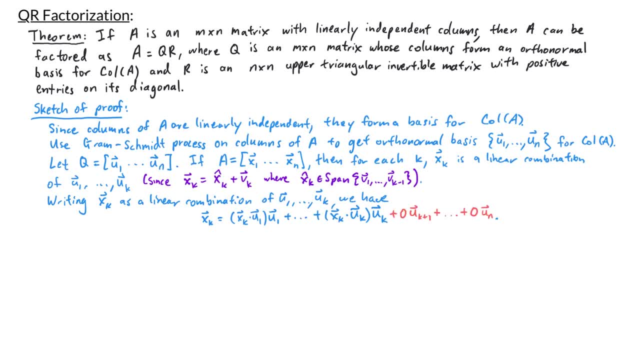 ued through un. so we must have that. the weights for the vectors uk plus one through un are all zero. now let r be an n by n matrix with columns r1 through rn, and let's say each of the columns rk have entries r1k, r2k through rnk. now if i take the product of q and r, i would have the product. 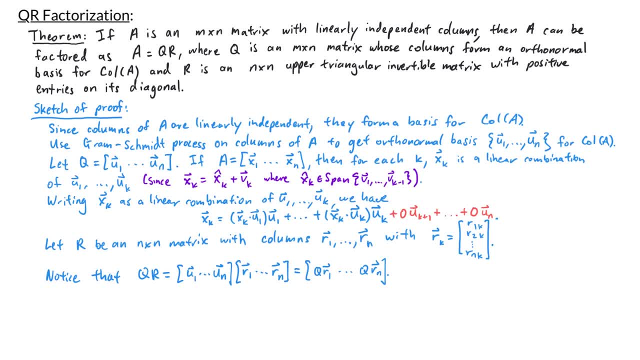 of the matrix u1 through un times the matrix r1 through rn. this can be rewritten as the matrix with columns q times r1 through q times rn. so if a is equal to q times r, then we have that the matrix with columns x1 through xn is equal to the matrix with columns q r1 through q? rn. so we need: 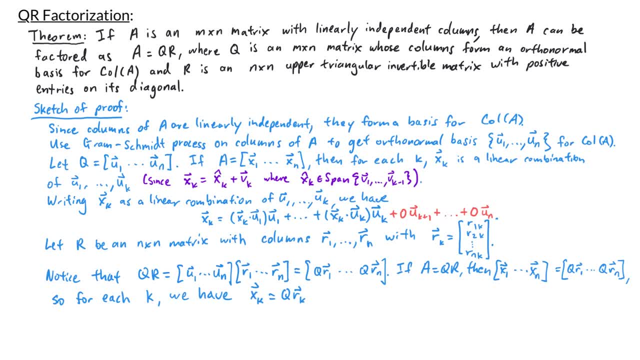 that each xk is equal to qrk. But if I multiply out qrk then I have a linear combination of the vectors u1 through un with weights r1k through rnk. From above we know how to write xk as a linear combination. 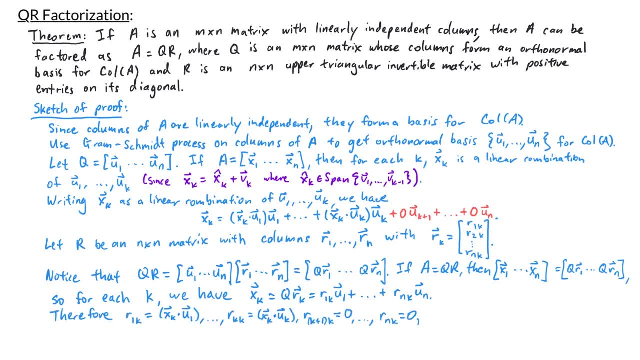 of u1 through un. so equating the weights, we have that r1k must be equal to xk dot u1, and all the way through to rkk would equal xk dot uk and then afterwards rk plus 1k. 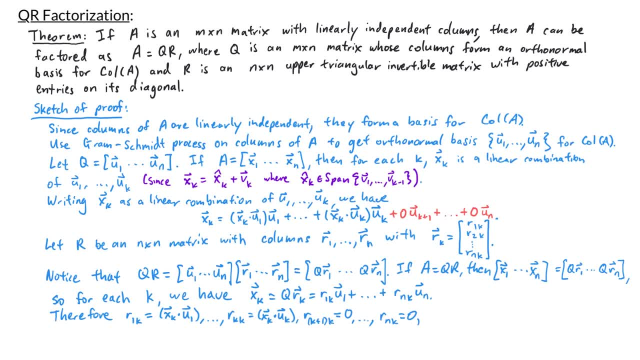 would be equal to 0, through to rnk would also be equal to 0. So in the end our matrix r looks like this upper triangular matrix. Again, we know that this matrix is upper triangular because when we write xk as a linear combination of u1 through un, we have the weights for: usk and the vectors xk and others in here will have the heights of qrk and the forces will then be eaten by qrk and the vector Q. Notice that the k will be equal to stressing out qm3, because u1 is a linear combination of xk. So again, this sen based on this matrix. 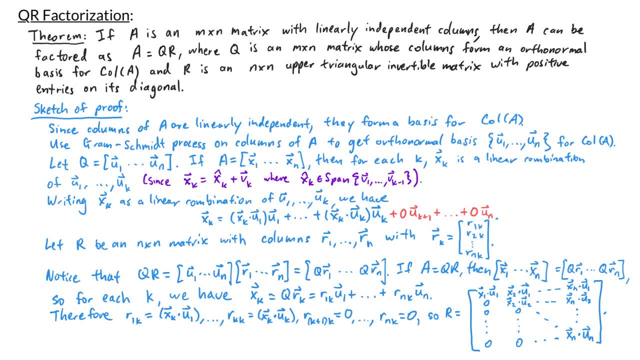 u k plus 1 through u n are all zeros. We also know that the entries along the diagonal are positive because I can write x k equal to x k, hat plus v k, And the v k here is just replaced by u k times the length of v k. So that's why the diagonal entries are positive. Lastly, since r 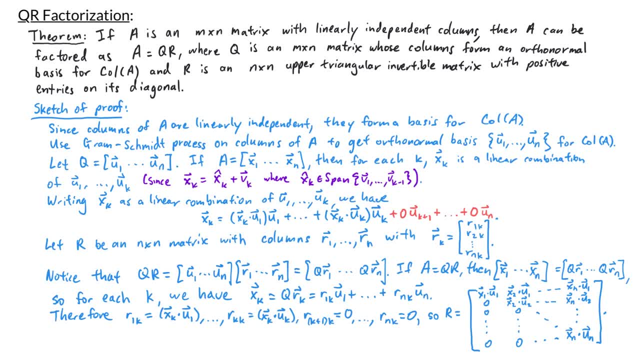 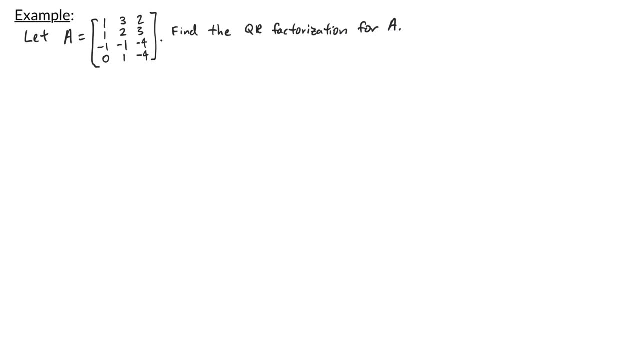 is a triangular matrix with non-zero diagonal entries. I know that r is invertible, So hopefully this gives you a rough idea of how this theorem is proved. Now let's look at an example of finding the qr factorization for a matrix. In this example we have the matrix A, given by 1, 3, 2,, 1, 2, 3,. 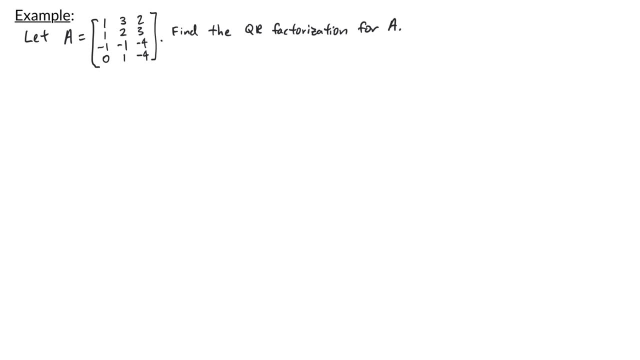 negative, 1 negative, 1 negative 4, 0, 1 negative, 4.. And we're asked to find the qr factorization for A. Before we start, I want to mention that once you have the matrix Q, it's very easy to find the qr factorization for A. 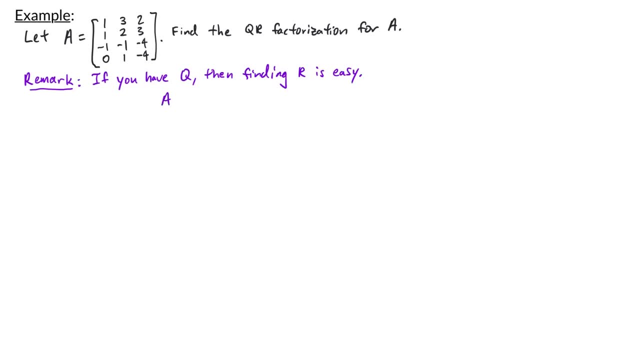 Because if I have A equals q times r, what I can do is multiply both sides of the equation on the left by q transpose. Now, in a previous video we've proved that if I have a matrix with orthonormal columns, like we have in this case for Q, then q transpose Q is just the n by n. 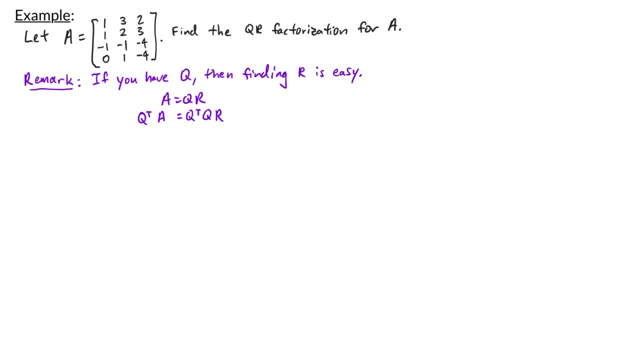 identity matrix. So on the left there I'll have q transpose A, and on the right I have the identity matrix times r, which means r is just q transpose times A. So now let's return to our example. So here the columns of A are: x1 equals 1- 1 negative, 1- 0,. x2 equals 3: 2 negative, 1- 1,. 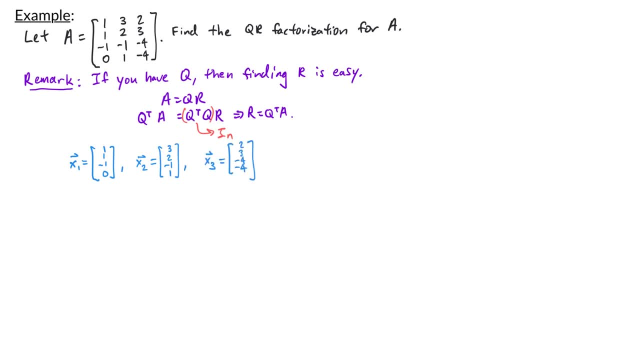 and x3 equals 2, 3 negative, 4 negative, 4.. If I want to find Q, I would need to use the Gram-Schmidt process on these columns to find the orthonormal basis for the column space of A. Luckily, we've. 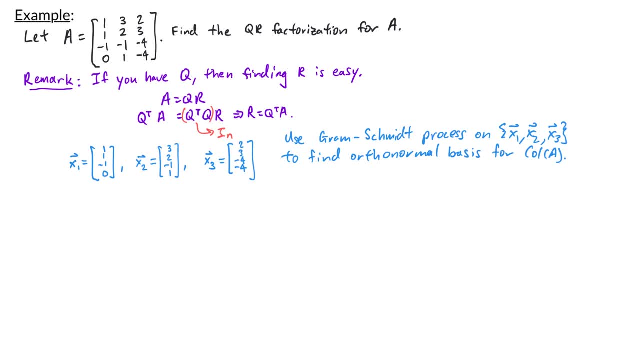 done this in our last video, We found that an orthonormal basis for the span of x1, x2, x3 is the set: u1 equals 1 over root 3, 1 over root 3. negative 1 over root 3: 0.. u2 equals 1 over root 3, 0, 1 over. 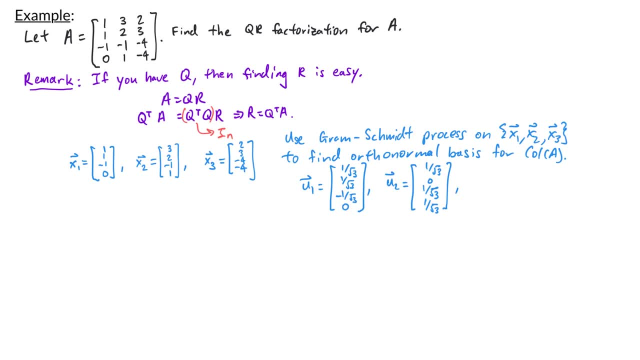 root 3, 1 over root 3.. And lastly, u3 equals 1 over root 6, 0, 1 over root 6 negative, 2 over root 6.. So q is the matrix with columns u1,, u2, and u3.. And again, to find r, we just do q, transpose times A. 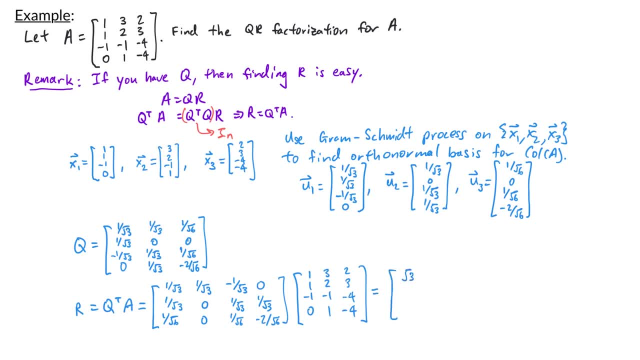 Multiplying this out, you get: r equals square root of 3,, 2 square root of 3,, 3 square root of 3,, 0 square root of 3, negative 2 square root of 3, and, lastly, 0, 0 square root of 6..